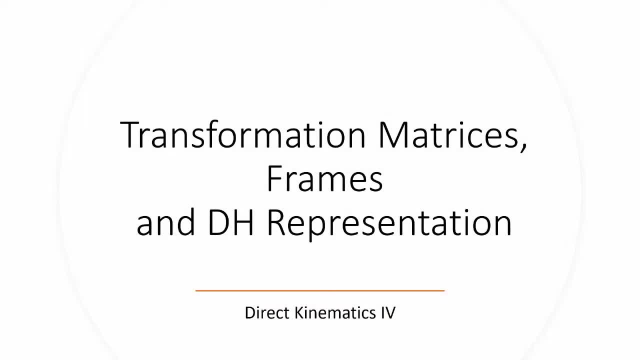 Hi everyone. in this video we are going to be going through a worked example encompassing everything we've learned thus far, which would be assignment of frames, DH tables and, finally, transformation matrices. So let's get into it. If you guys like this video, don't forget to give me a thumbs up and 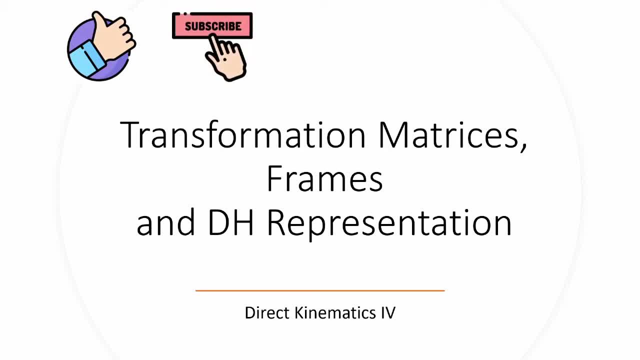 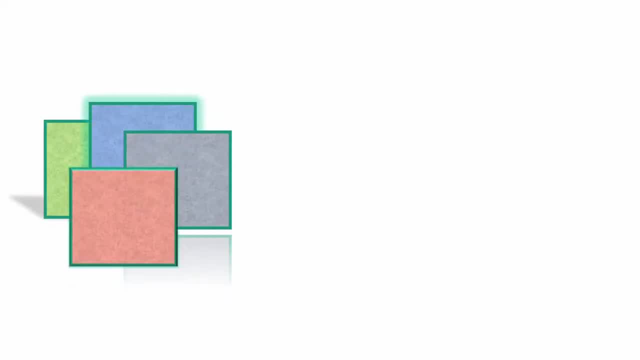 please subscribe. I'm Trumps and welcome to That's Engineering, Alright, guys. so this is a robot that we will be looking at Now. forgive my sketching, I know it's not perfect, but what I've tried my best to show you is a robot with three revolute joints, where this would be the first. 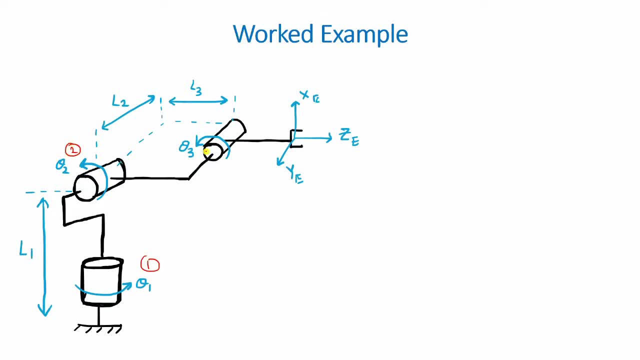 joint. this would be the second joint and the third joint, each having their own angle of rotation. theta L1, L2, L3 would be the distances or the link parameters, and this would be the tool which already has its frame pre-assigned. now there are four steps that we will be looking at, the first being frame assignment and 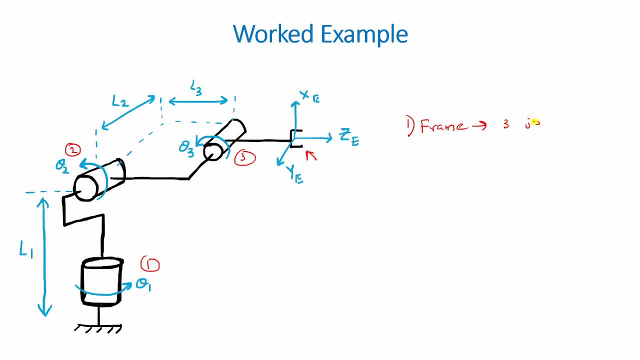 this will be done for the three joints. from this we will look at making the DH table and from the DH table the transformation matrices. and this can be done using equation we have learned. and from the transformation matrices we can do any matrix allocation algebra to find any unknowns that we don't know. in this case we look for T E. 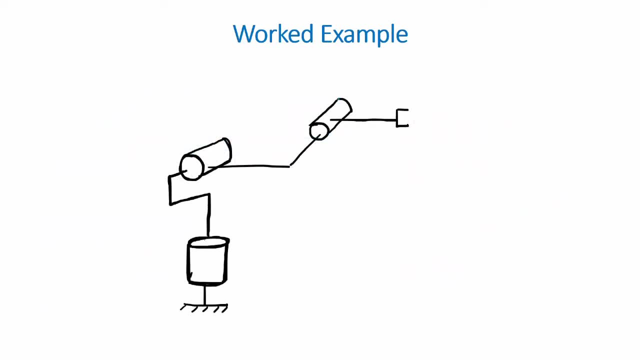 13. alright, the first step would be frame assignment. she'll be using the 6 conventions we learned and we'll start off with identifying the joints and their joint axes. so we have to first ever do joint here, second revolute over here and the third joint over here. The first would have a joint axis sort. 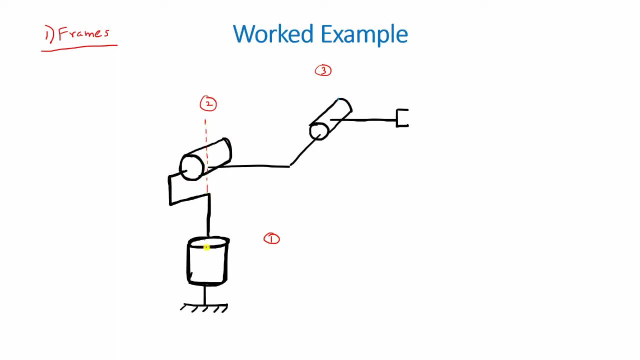 of something similar to this, running vertically. the second would be here and the third would be here. Now, something to note is that joint 2 and joint 3 are actually parallel to each other. just that, the way I've drawn it, it looks slightly different. Now we can assign: 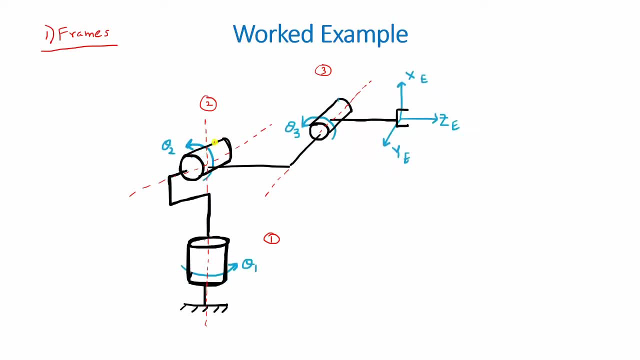 the direction for each of the joint axis by considering the theta value. and to do this we would look at our right hand rule, where the direction of the fingers would point in the direction of theta and the thumb would show where the positive axis is. and if you use this for joint axis 1, it should point in this direction. 2 would 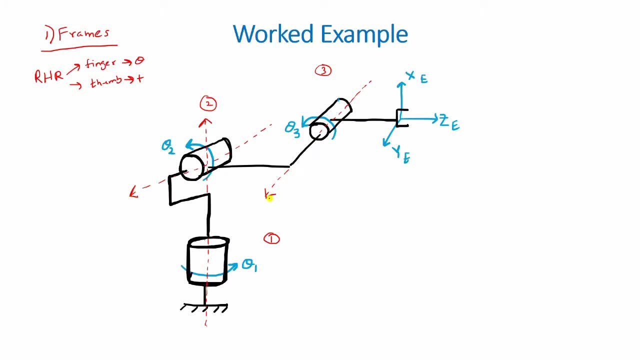 be in this direction and 3 would also be in this direction. We can now assign our z axis to our 3 joints, so we would have z1, z2 and z3.. The next step would look at assigning the origin for each of our joint axes. 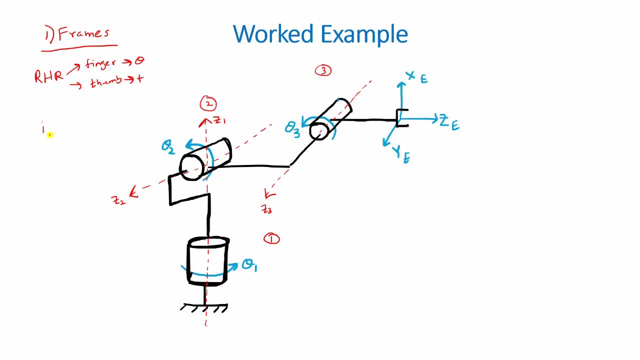 Now again, we will consider i and i plus 1. so when we look at joint 1, we consider joint 2.. As the two joint axes intersect, the point of intersection becomes the origin for the first axis. So z1 will intersect at this point, and so this would be the origin For 2 to 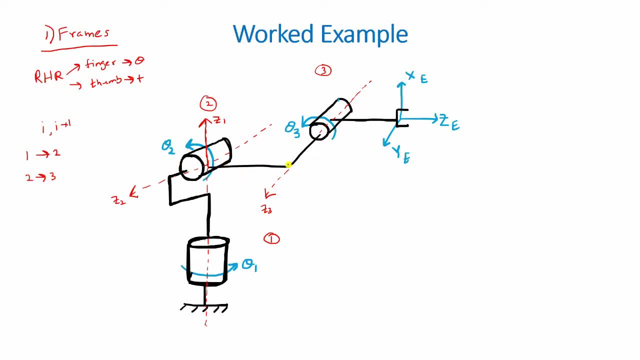 3. Since they are parallel, we will look at the common perpendicular which lies along this particular link. Therefore, the origin of z2 would be the start of the common perpendicular, which would be the start of the link. So z2 would lie in this direction. 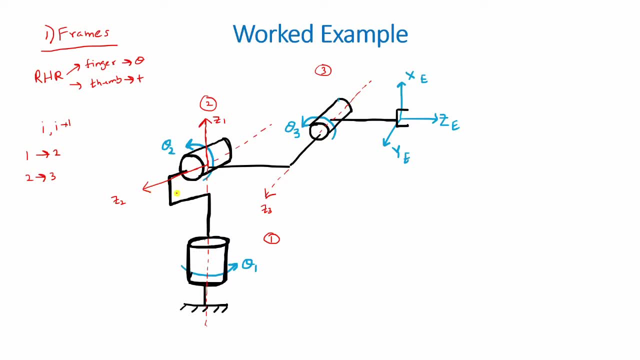 Right then to set z3, we will consider the next frame, which is the tool. Here. they are both intersecting with each other. as ze has this sort of joint axis. The intersection point is over here, making that the origin for z3.. Right then to set z3, we will consider the next frame, which is the tool. Here they are. 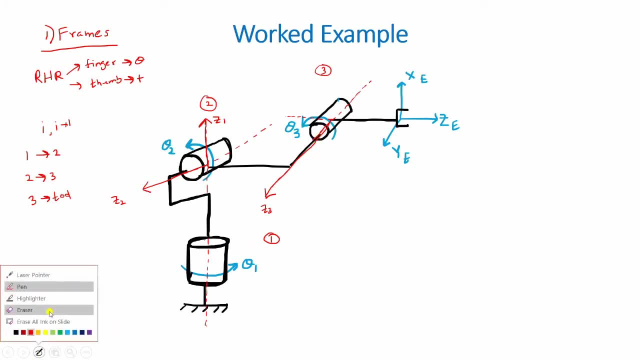 both intersecting with each other. One is z3 and the third, x, is z2 due to the constant right. Alright, so now that the z axis and the origins have been set, we can look at setting the x axis. Now, if the two axes intersect, we look. 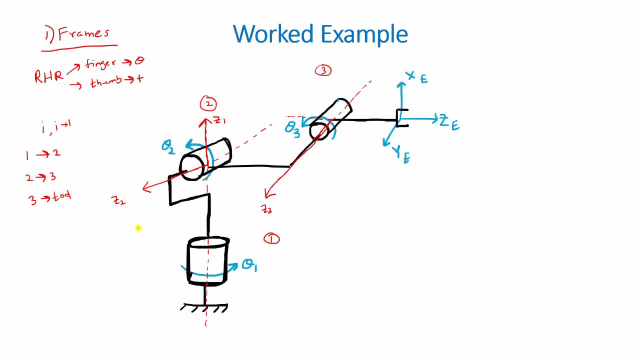 at the intersection of the planes and the x axis would be normal to that. if, however, the axes are parallel, x would lie along the common perpendicular. Henceforth we look at the planes, So the plane here would be something like this: So if I draw it out separately, you will have one plane here. 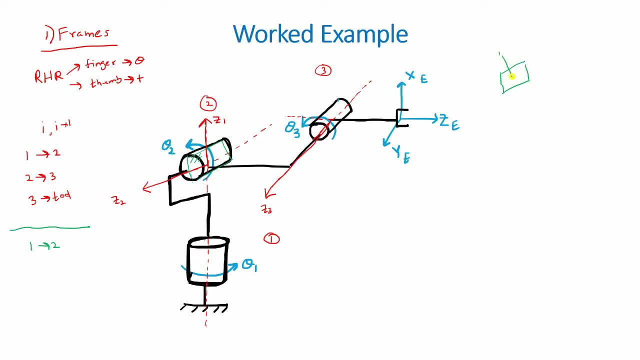 and another plane over here, and so X would be normal in this direction and That just so happens that it is along the link, This link, so X1 Would be along this particular link. now, from 2 to 3 They are parallel to each other, So X2 would lie along the common perpendicular. 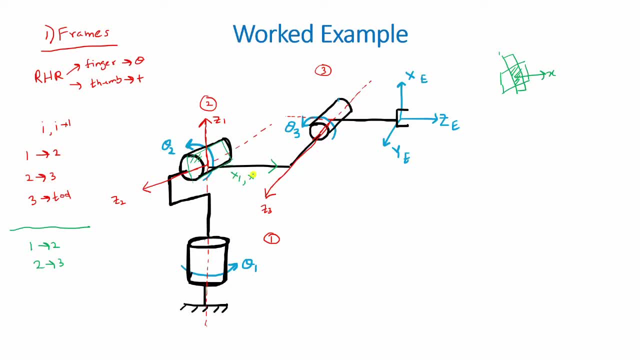 Which also happens to be at the link. so X1 and X2 would coincide with each other along the link From 3 to the tool. Here again the two axes intersect, so it's a point of intersection. So we look at the intersection between the two planes in this case. 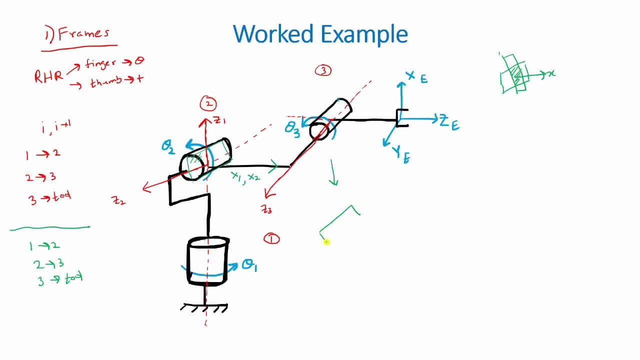 The z3 plane would look something like this, While the ZE plane would look something like this. So this area Pointing upwards would be the x-axis. So therefore, from this point x-axis Would point upwards X3. So again you can see that x1 and x2 are sort of opposite to the direction of rotation. theta 2. 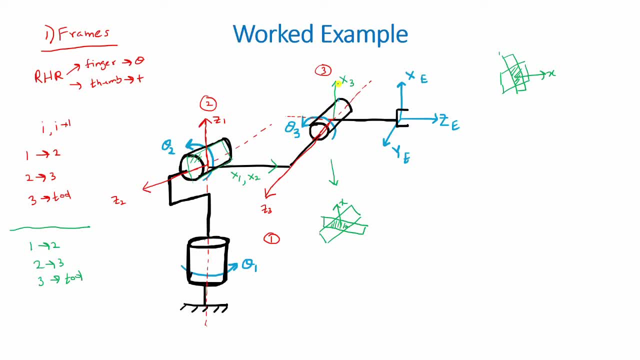 While x3 is opposite to the direction of rotation theta 3.. That is why we know it points upwards. Now we don't really need to find the y-axis, because it's not needed for the calculations. the frame for the tool is already given. But what we can do is find the base. 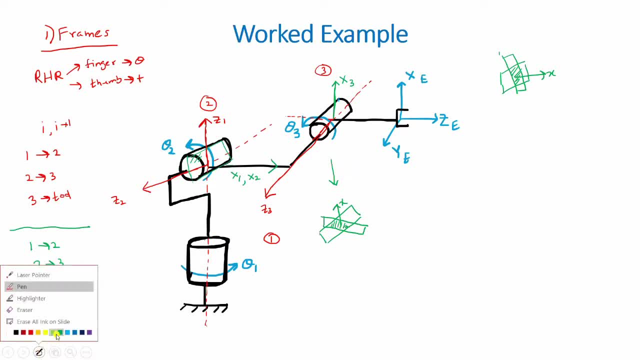 frame Right. so this marking here shows that this is the base frame. So we can assume the origin of the base frame would be at this point. We will assign the base frame arbitrary, but we will do so to closely match the first frame. So Z naught. 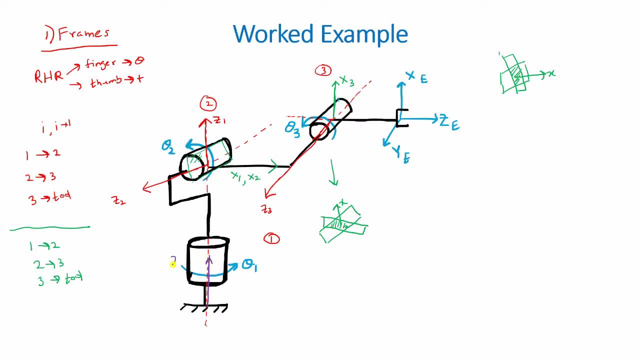 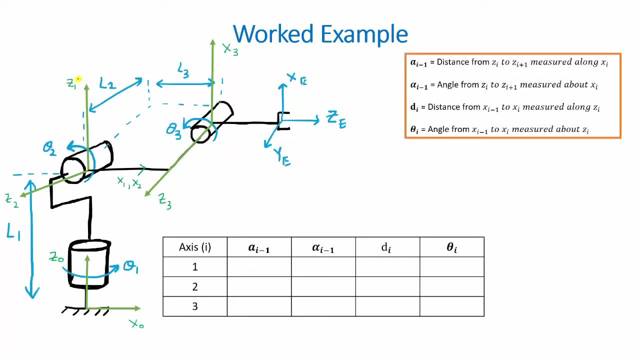 would be along here and X naught would be In this direction. Alright, so the second step would be to find the DH table Using our four link joint parameters. Here, when considering the axes, we move on one to the other, so we would go from 0 to 1. 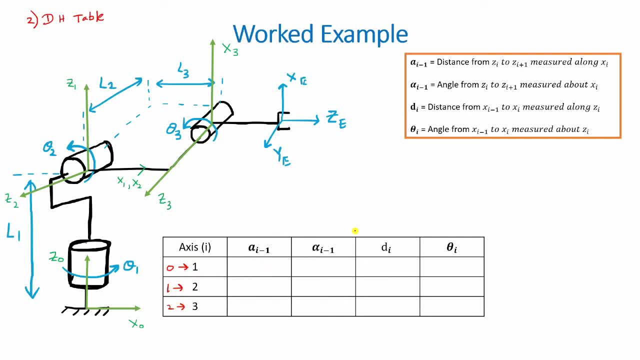 1 to 2 and 2 to 3. So considering the first case, 0 to 1- for the first two parameters I would be equal to 0 and For the next two parameters I would be equal to 1. So for a I minus 1, we would want the distance. 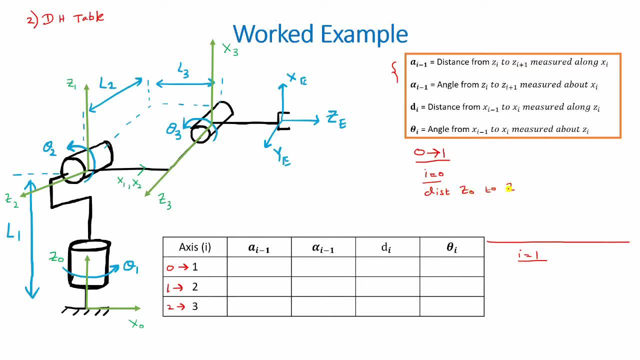 from Z naught to Z 1 along X naught. So the distance between Z naught and Z 1 along X naught would be 0, as they are both on the same line of action. For our alpha I minus 1, it would be the angle between Z naught and Z 1. 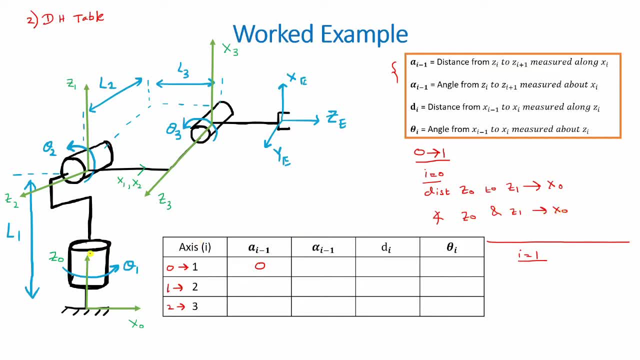 About X naught. So as both Z naught and Z 1 are pointing in the same direction, The angle would be 0, because it would look at the angle that Z naught has to rotate by to match up with Z 1, Then The distance. 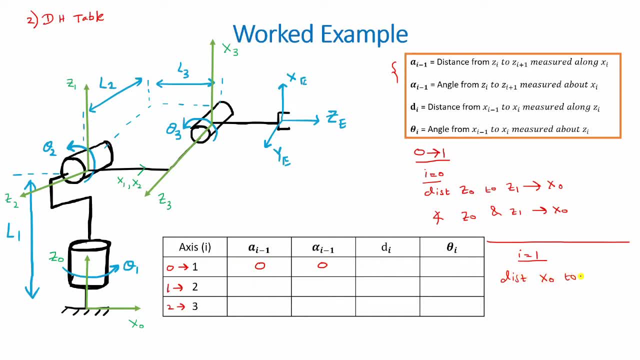 Between X naught to X 1 Along Z 1, So the distance from X naught to X 1 in the Z 1 direction would be L 1. Now this value would usually exist if it was a prismatic joint, but in this case it's a revolute joint. 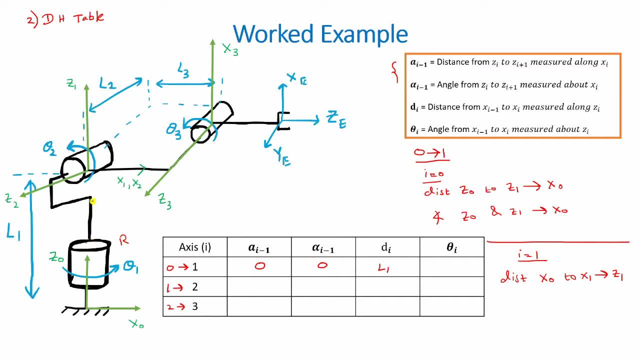 However, the value still exists due to the offset created by the link structure and The final value would be the angle between X naught and X 1 about Z 1. So if X naught was stationary, X 1 could rotate In relation to X naught about with an angle theta 1.. So this value would be theta 1. 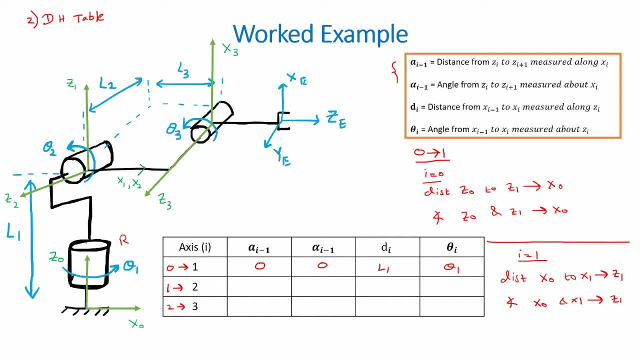 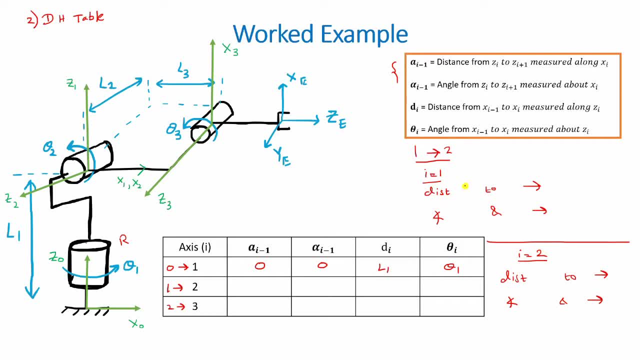 So for a I minus 1, we would want the distance between Z 1 to Z 2 along X 1, So the distance Z 1 to Z 2 in the X 1 direction would be 0, as they both have the same origin. 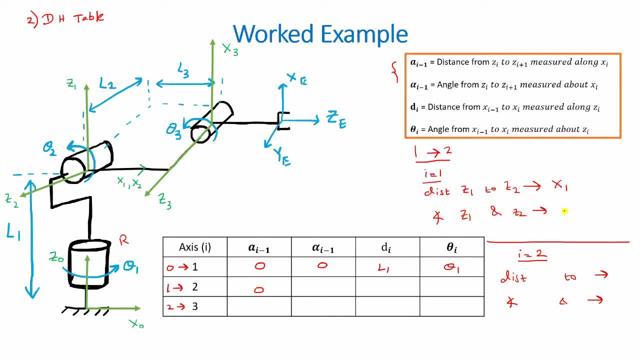 Then the angle Z 1 to Z 2 about X 1. So in this case the angle Z 1 must rotate to match up with Z 2. if rotated about the X 1 axis, Which is in this direction, and Z 1 would actually have to rotate. 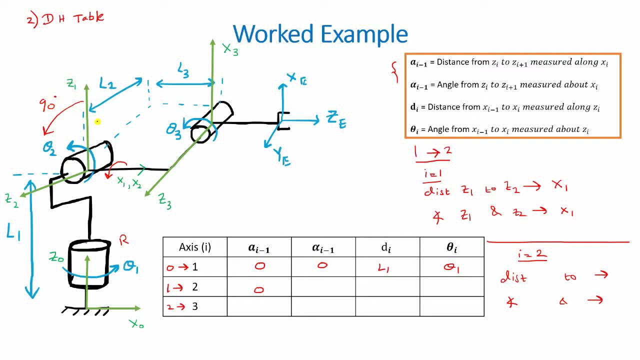 by this amount, 90 degrees. So it's actually 90 degrees counterclockwise. So because of that, it's positive. So the usual convention that we use Is if we have a counterclockwise rotation, it's taken as being positive, While a clockwise rotation is taken as being negative. This is just a convention that we normally use. 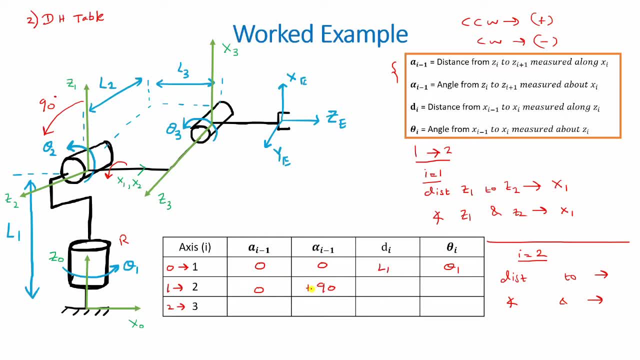 So that's why the sign here would be plus 90 degrees. Right for I equals 2. we want the distance from X 1 to X 2 about Z 2. So in the line of Z 2, the distance or the offset of X 1 and X 2. 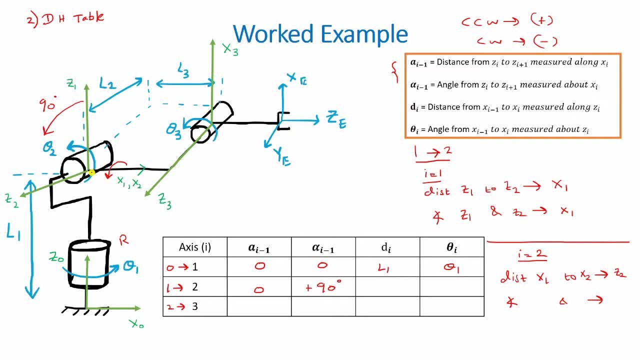 they're both on the same line and they both have the same origin, so this offset would be 0. and Finally we have the angle X 1 and X 2 about Z 2. So that is, if X 1 is stationary, how much X 2 can rotate about Z 2, and the value for that would be: 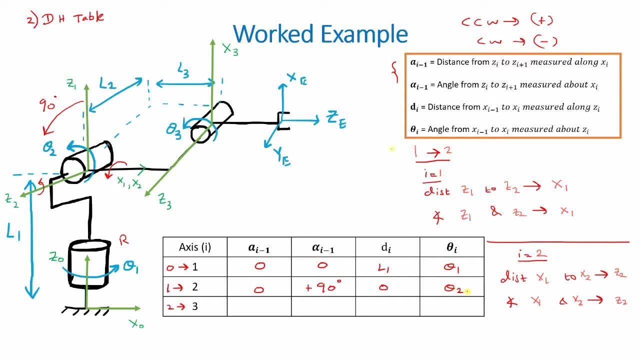 theta 2. Right. so now let's have a look at the last set of axes, Which is from 2 to 3. for the first two parameters, I would be equal to 2, and then I would be equal to 3. for AI minus 1, we want the distance of. 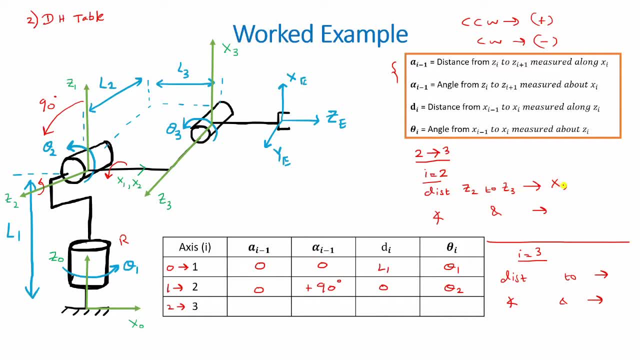 Z 2 to Z 3 about X 2. So that is the distance between Z 2 and Z 3 in the X 2 direction, And that distance will be the length of this particular link, which is L 3. Then for alpha I minus 1, the angle. 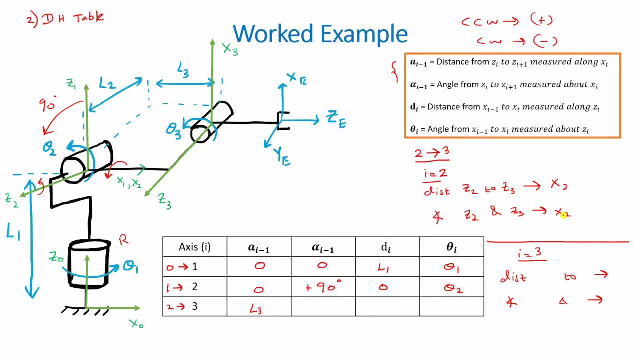 Z 2 and Z 3 about X 2. So that is the angle That X 2 would have to rotate to match up to Z 3. I'm sorry, the angle Z 2 would have to rotate to match up to Z 3 if rotated about X 2. 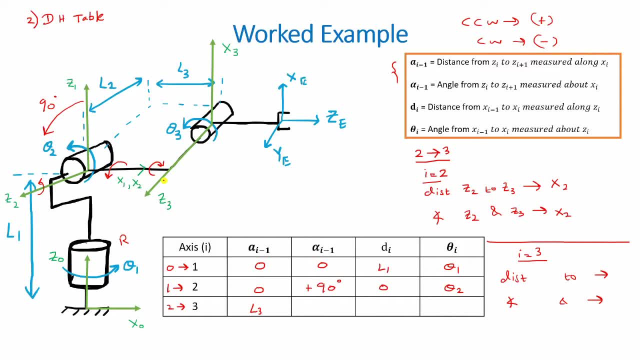 That is, anywhere in this direction. as they are both pointing in the same line and are parallel to each other, This angle would be 0. For the next two parameters for di, we look at the distance between X 2 to X 3. About Z 3. 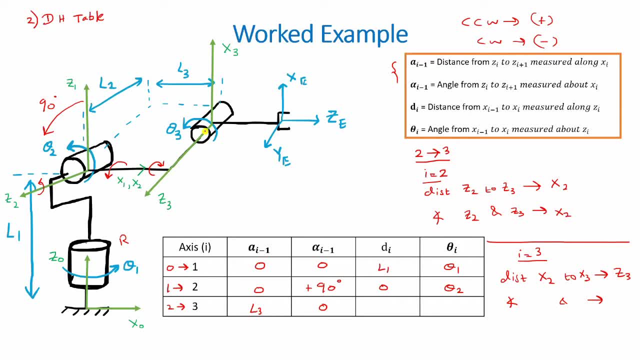 so the distance between X 2 over here and X 3 over here in line of Z 3, so this distance would actually be the length of this Particular link over here, which is L 2 as given, But Z 3 is pointing in this direction. 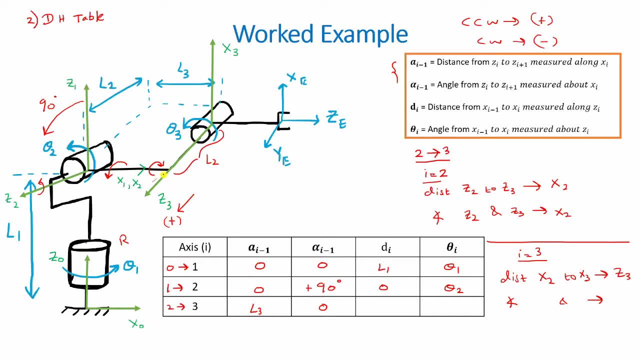 Which means this direction is positive. and since we're moving from X 2 to X 3, we are moving in the opposite direction, So this value would be negative: L 2. The final one is a bit tricky, but let's have a look at it: the angle between X 2 and X 3. 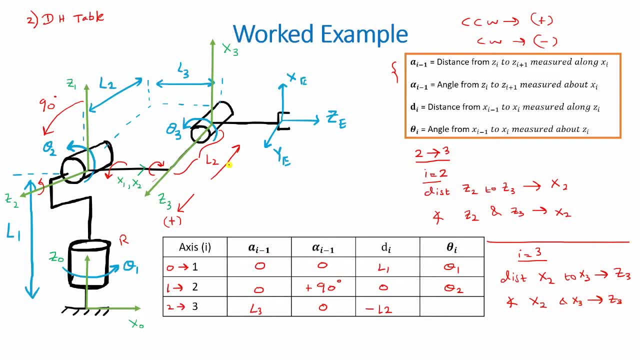 If rotated about Z 3. So first of all, let's have a look at it. Z 2 stays stationary and if Z 2 is stationary, Relative to that, X 3 can rotate by some angle- theta 3, So we have a theta 3 term here. 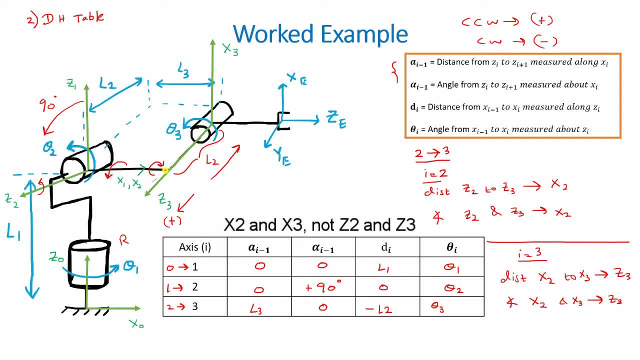 In addition to that, the amount Z 2 has to rotate to match up to Z 3 about the Z 3 axis would be 90 degrees and In this direction, because they both have to point upwards. So in addition to the rotation of theta 3, there is an extra 90 degrees and this is true if you look at it again. 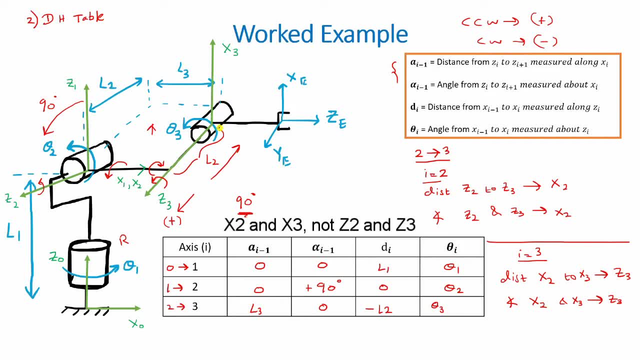 You have Z 2, which can rotate 90 degrees to match up to Z 3, and then Z 3 can rotate further by theta 3 degrees. So theta I in this case would be theta 3 plus 90 degrees, And that is the DH table. 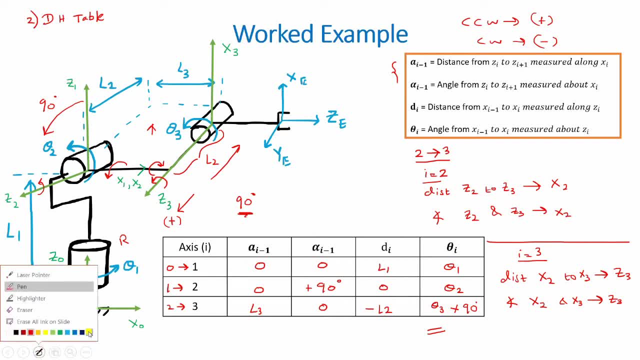 so something to note from here is That if you have a rotation, You will look. if the rotation is counterclockwise, It would be positive, if clockwise it would be negative, and this is purely by convention. the second would be: if you want to identify if a rotation is clockwise or anti-clockwise, you would look at it and 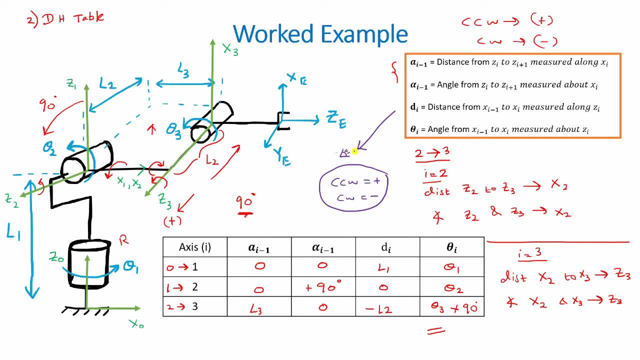 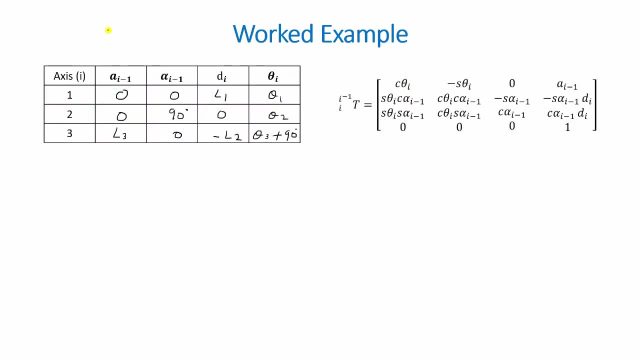 From over here, So by looking at it from this side of the axis, a rotation in this way would be Counterclockwise, while the rotation in this direction would be clockwise. Alright, so the next step, which would be the third step, is to find the transformation Matrices. 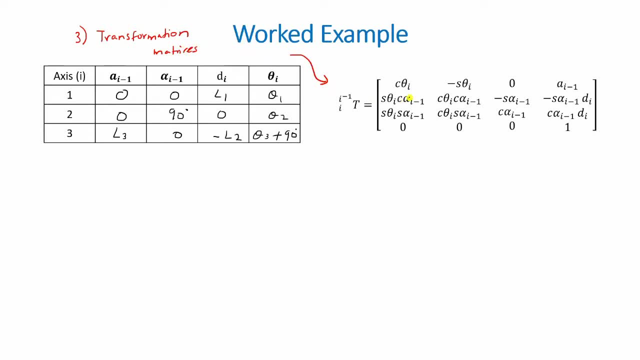 And this can be done using this equation, where you can directly plug in the values and find your transformation matrices. so first we have T 0 to 1, because we moved from x's 0 to 1, 1 to 2 and 2 to 3, so the T 0 to 1, we will use the first row from our DH table. 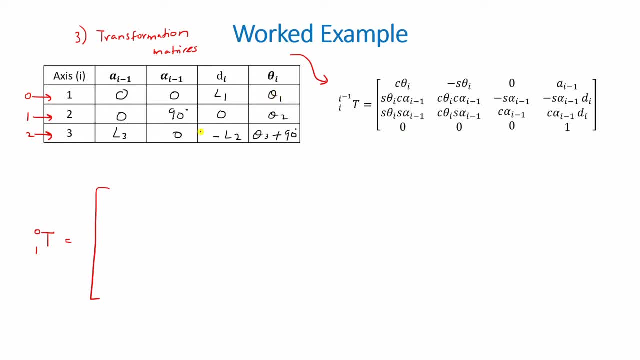 Okay, you have cos theta i, which would correspond to cos theta 1. then it would be minus sine theta 1: 0. a I minus 1 is also 0, right? second value: sine theta 1 cos 0. so it would be sine theta 1 when simplified, and this would be cos theta 1. you will have: 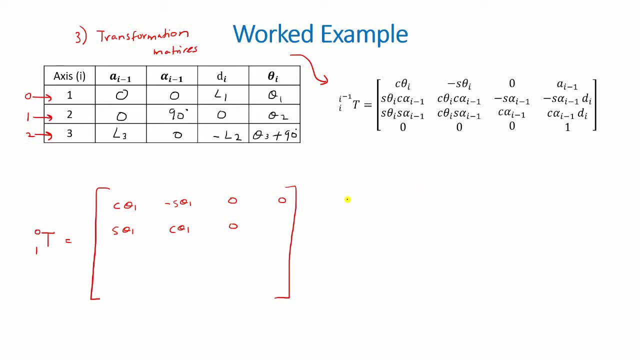 0 cos sine 0 is 0 and the second value would also be 0, again 0 sine alpha. I minus 1 is 0, so this whole term goes to 0, this whole term goes to 0, this term would become 1 and this term would: 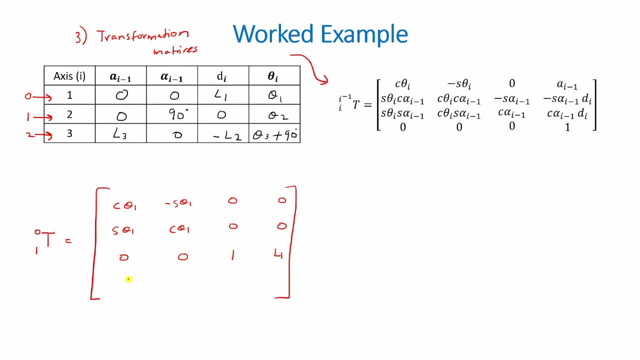 become L 1, because di is equal to L 1 and 0 0 0 1. so, again, as we saw in the first few videos for this playlist, this is a rotation around this Z axis and shows the orientation of the manipulator, while this shows the position of the manipulator. 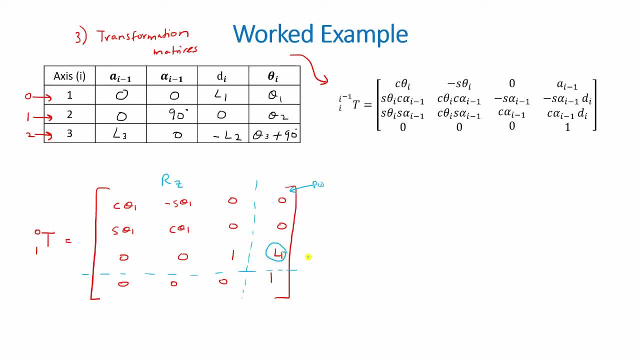 and you can see this term. L 1 here is on the Z axis. you have your P X, P Y and your P Z and this matches up because the first joint which was over here, the first joint which had its origin somewhere here, was L 1 away from the base in the Z direction. so that is why this L 1 is over here. so it makes 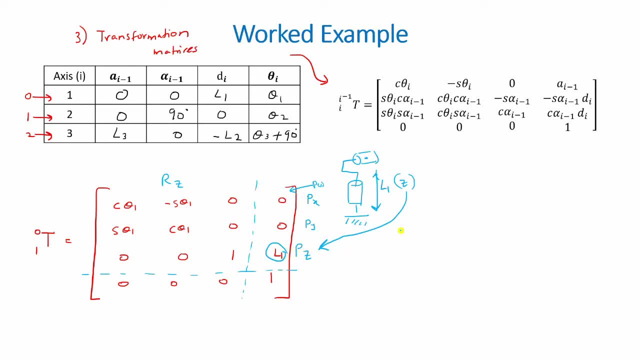 sense. now let's learn about the quantum matrix again and if we go back to the previous video, so have a look at T 0, 2, right T. so it would be 1 to 2, right T: 1: 2. we use the second row values, so cos theta 2 minus sine, theta 2: 0 a I. 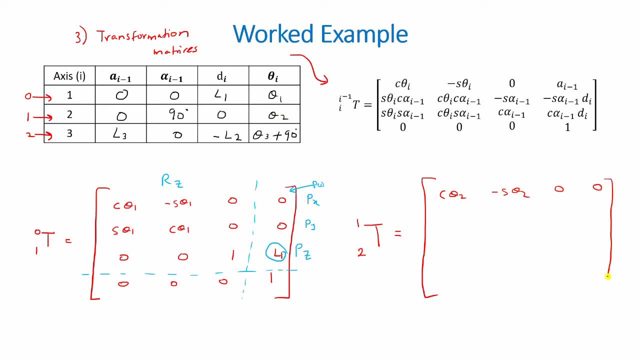 minus 1 is also 0. then we have sine theta I, which would be sine theta 2, into cos alpha I minus 1 would be cos 90, cos 90 would be 0. so this term goes to 0. this term goes to 0. 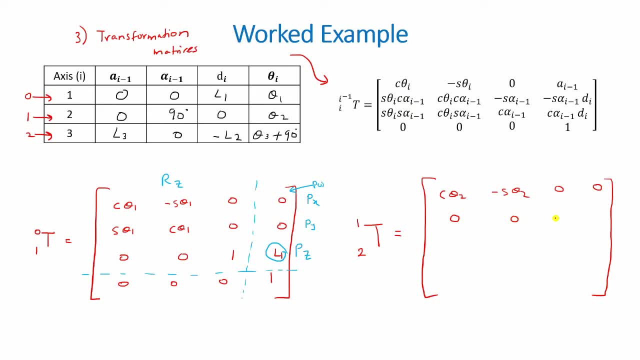 minus sine 90 would be negative 1 and this would be 0, because di is 0 here. sine theta I would be sine theta 1, sorry, sine theta 2, while sine alpha I minus 1 would be 1. so sine theta 2, cos theta 2, cos 90, 0, cos 90, 0 and 0 0, 0, 1 right. 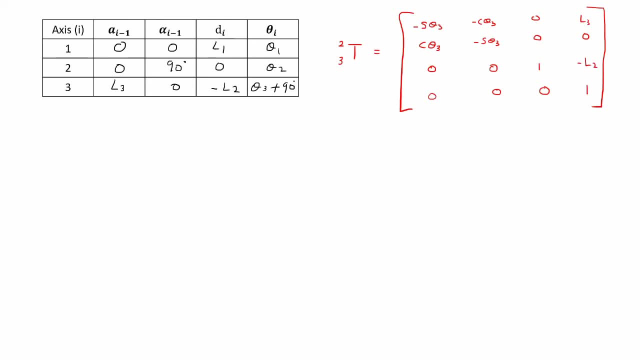 right. so you can solve in a similar manner for the last set of axes, which is 2 to 3, and you would actually have theta 3 plus 90 degree terms, for example cos theta 3 plus 90 and sine theta 3 plus 90. and if you were to 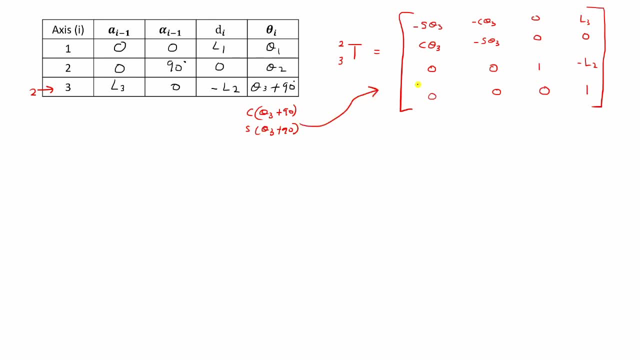 simplify all these terms, you should get this matrix for transformation matrix of 2 to 3. the next step, which is the final step, wanted us to find the transformation matrix 0 to 3, and we can do this by simply multiplying 0 to 1, 1 to 2 and 2 to 3, which is what we found in the previous part.